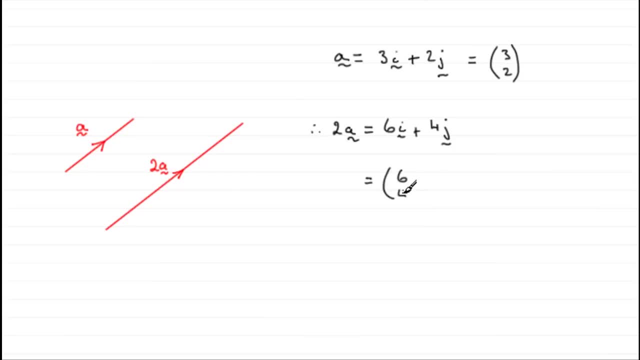 column vector simply 2J, 6,, 4.. And we can do the same with vectors in three dimensions. If I've got a vector B which was 5I minus 2J plus 3K and I wanted to triple this vector, say 3B, 3B would clearly be 15I minus 6J. 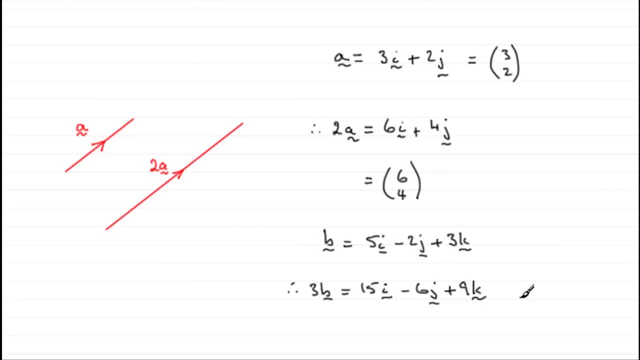 plus 9K and so on. Very easy idea. Now we can also do a vector with a vector B, which would be 3J plus 3K. So if I've got a vector B, addition of vectors, If we have two vectors, say A and B, when it comes to vector addition. 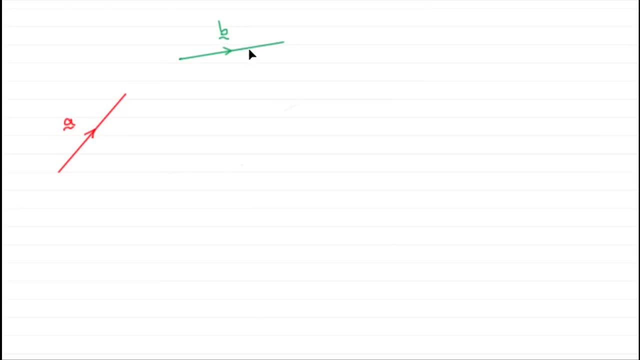 it's like taking our vector B and putting it on the end of A, So we have really what is called A followed by B, And this particular vector, A followed by B, is a vector from here to here, And it's called A plus B, A followed by B. It's not the normal addition that we 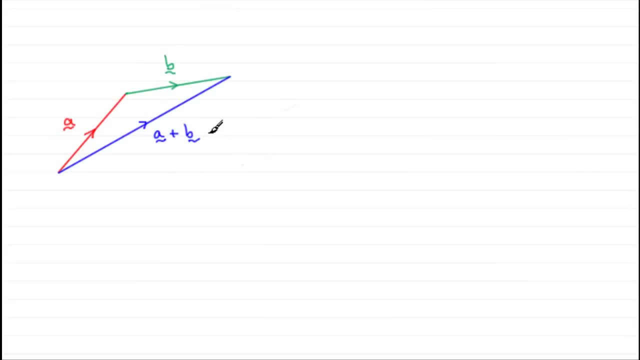 might think of when we do say 3 plus 2, which equals 5.. No, This is something different. Think of the plus as followed by. So we're doing this movement A followed by this movement B, And it's equivalent to going from here to here. So A plus B, We can also do subtraction. 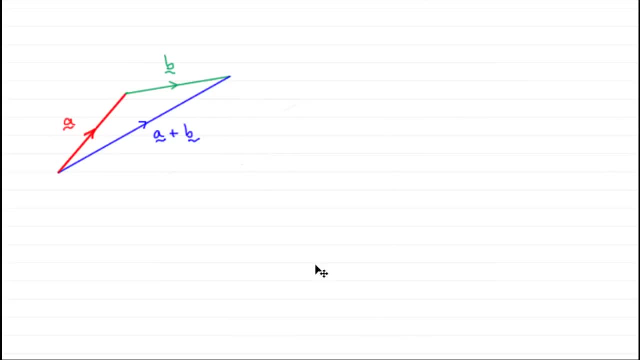 of vectors. We can also do subtraction of vectors. We can also do subtraction of vectors. Suppose we took our vector A and just moved it over here. Let's just write on that: that's the vector A. Now if we take our vector B but take the negative of it, that's this vector. 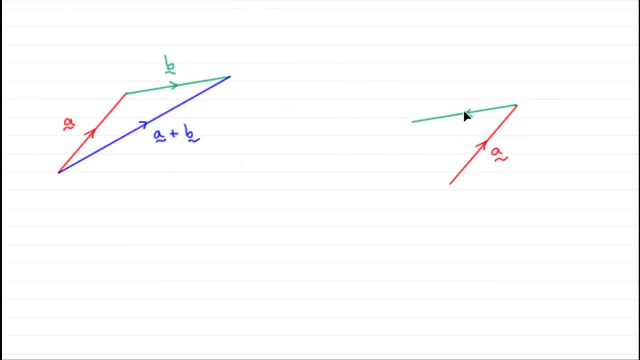 here, Bring it over to here and put it on the end of A. This vector, then, is minus B. We'll just write that on. It's going in the opposite direction, but it's the same length as B was. Then what we're doing is A followed by minus B, A plus minus B. It takes us from.